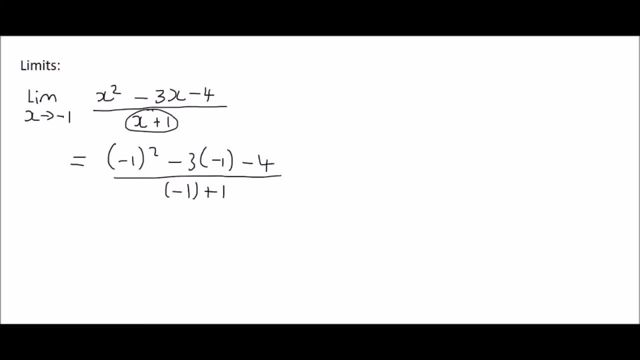 area that limits will catch you is when the denominator becomes 0. But then if you get a question like this, in the test it has been designed in such a way that the denominator can be cancelled, So let's see how that works. So now we're. 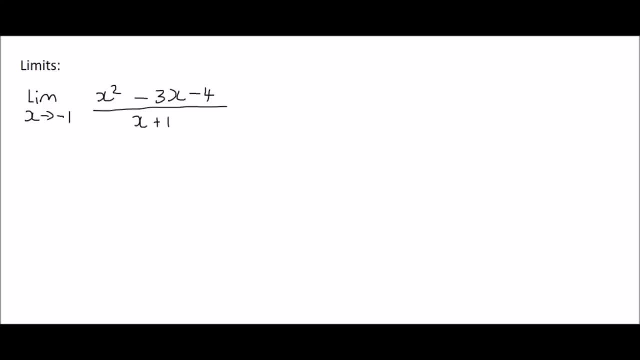 not gonna plug minus 1 in yet, So we're gonna carry on with the question. So now here's where teachers get very or the department is very strict about this. You have to keep saying equals to limit X goes to minus 1, and you have to keep. 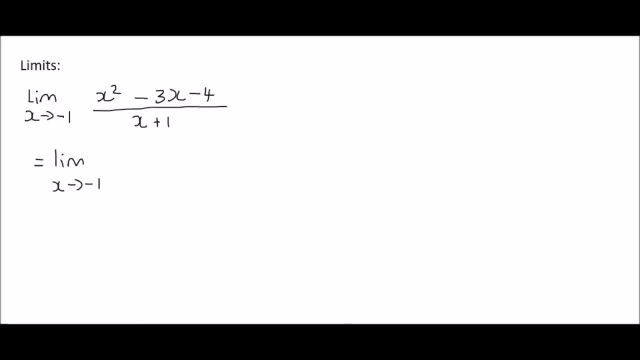 writing that until you actually use the minus 1.. And sorry if this doesn't, if this isn't clear what I'm doing here. it says X and then there's an arrow, and the arrow is pointing to minus 1.. So it says X is going to minus 1.. Okay, so now what? 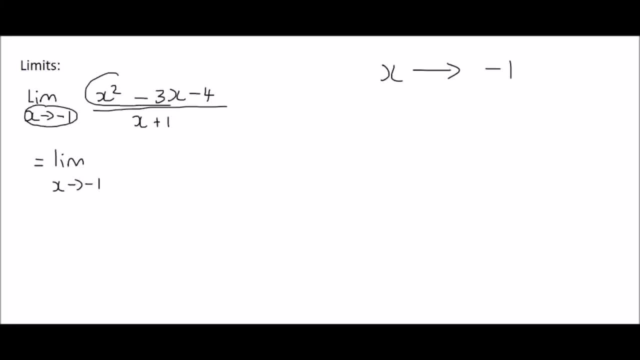 we're gonna do is we're gonna have to do a few things. So what could we possibly do at the top? Well, well done if you realize that we can factorize, and so that's a nice easy trinomial, They'll always design them as fairly easy. if 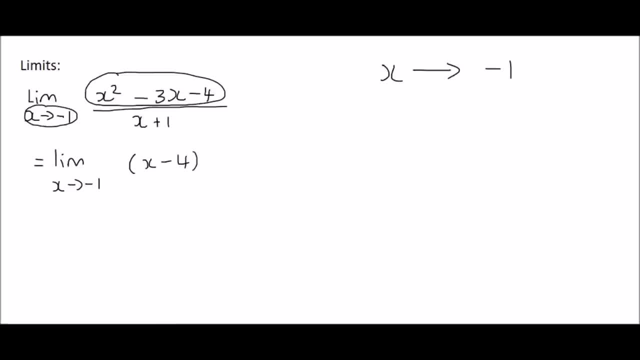 they need the denominator to cancel. So that's just gonna be X minus 4, X plus 1 over X plus 1.. And so that cancels, and so then we can just write: equals to lim X goes to minus 1 of X minus 4.. Now we can put the minus 1 into the equation, so then we can just 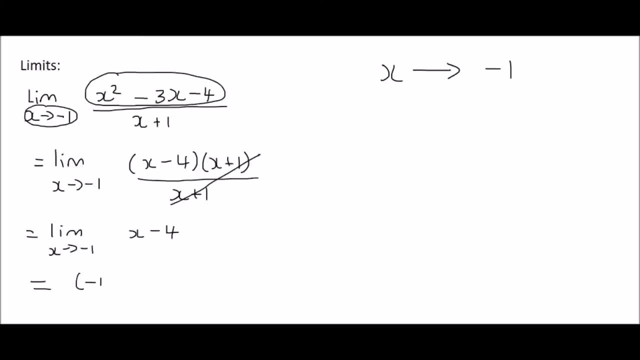 do this. Now you don't have to say lim anymore, because we're gonna use the minus 1 like that, and the answer is minus 5.. See, so it's easy. if you get an error on your calculator, then you just have to do an extra step and then just. 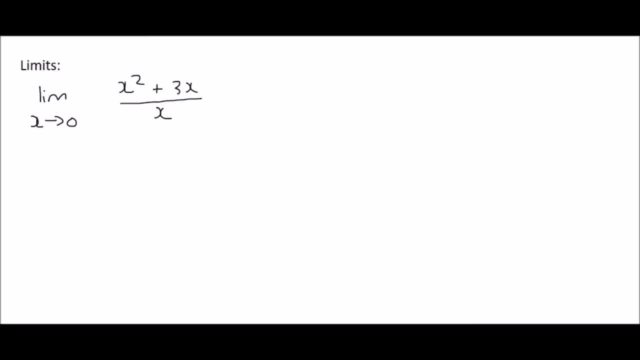 plug the value in. Okay, so here we can try plug everything in, but we can clearly see that there's a 0 at the bottom. and so if you just plug X- as sorry, there's an X at the bottom- and if you plug 0 into that, you're gonna end up. 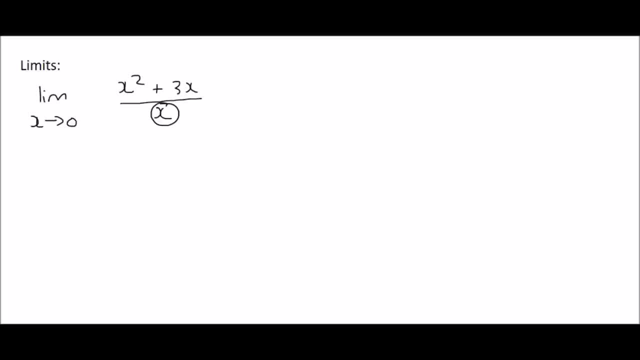 with a 0 and you can't have a 0 in the denominator. So then all that you do is you factorize. Then we're gonna have to say: equals to lim, X goes to 0. Then you take out X as a common factor at the top, and then you're left with X plus 3.. The 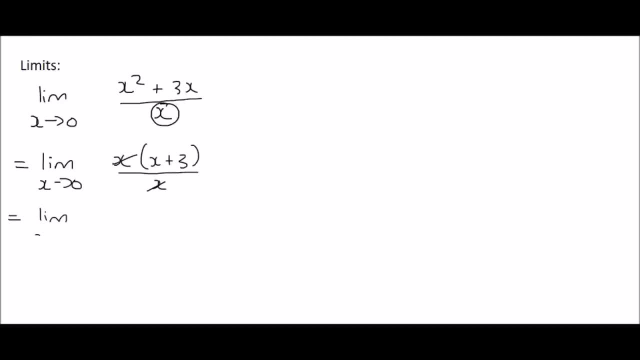 X's, then cancel, and so we can say: equals to lim X goes to 0 of X plus 3.. And now we can just plug the value in and so that's gonna give us 0 plus, so that's in bracket plus 3.. And 0 plus 3 is just 3, so the answer for that one is 3.. 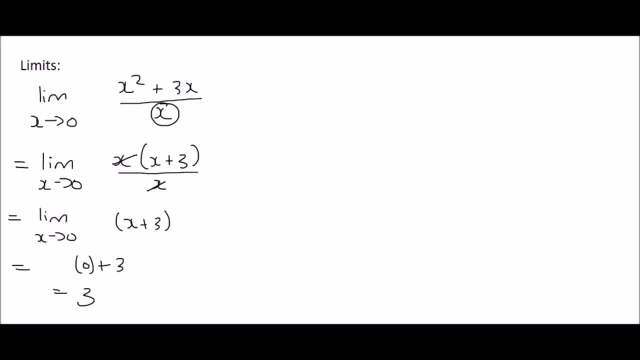 So, in summary, plug the value in if it doesn't work. factorize or do something that will help it to somehow. yeah, there will only be one or two things that you can possibly do. You simplify it like that and then you plug the value in and 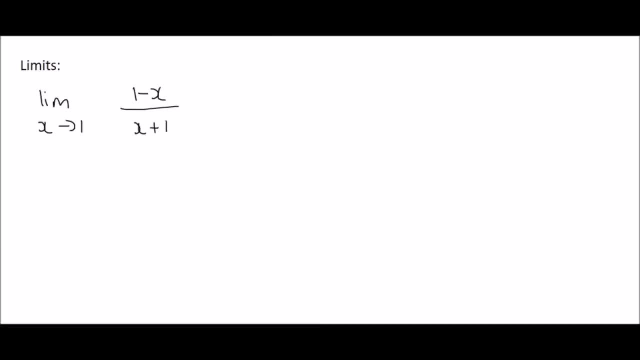 if you don't get an error at the bottom, you can just plug the value in to the error on your calculator. then it's all fine. here's another one. so we will start by just plugging the value in, and if you plug it in at the, if you plug one in at the top, you end up with one minus one. 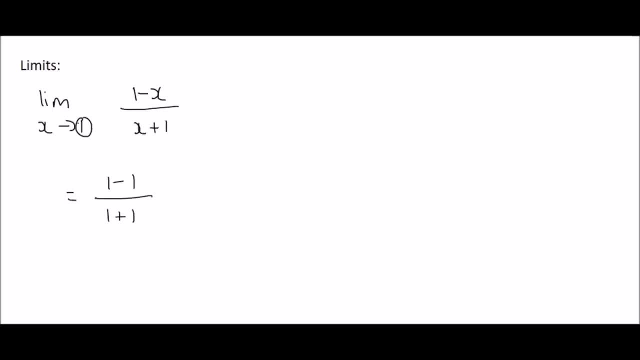 but then at the bottom you end up with one plus one. now this is okay, because we end up with a zero at the top, but a two at the bottom. that's fine. zero divided by two is just zero. what you don't want is you don't want a zero at the bottom. that's where the error comes in on the calculator. 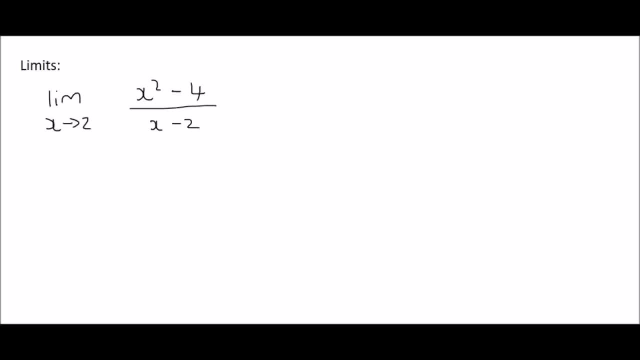 and that's when you're going to have to do something else. and here's one last one. so if we plugged two into this expression, well, at the bottom you would have two minus two, which is zero. now that's a problem, and your calculator would have given you an error. so then we have to. 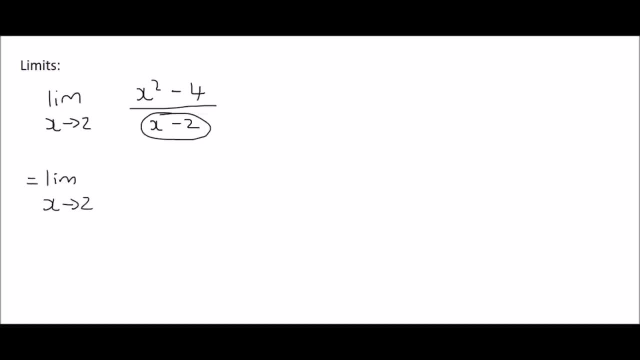 do a few things. so now, because we're not using the two yet, we have to keep writing this limb. x goes to two. that's very important. then at the top we have a difference of square, so it can become x minus two, x plus two over x minus two. those can cancel. 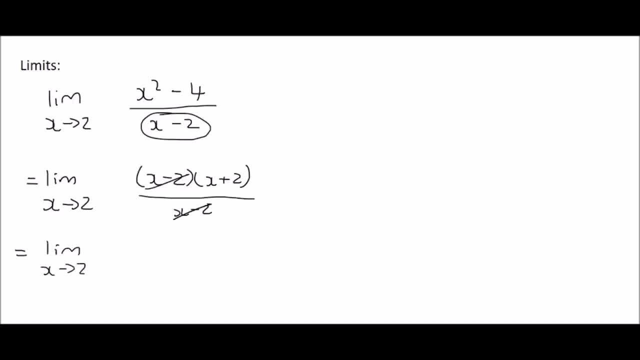 and so we're still not using the two yet, and that's gonna say x plus two. now we're gonna use the two, so we don't have to write lim anymore. so we just say two plus two, and that's gonna give us four.